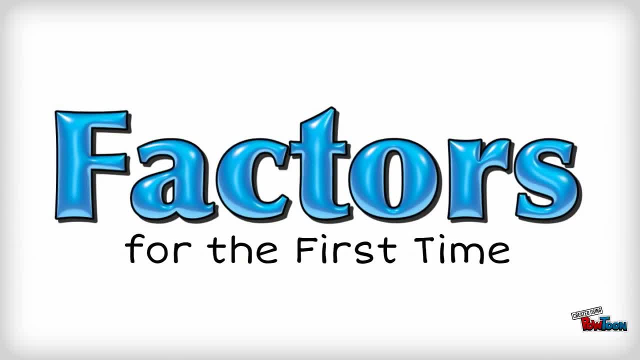 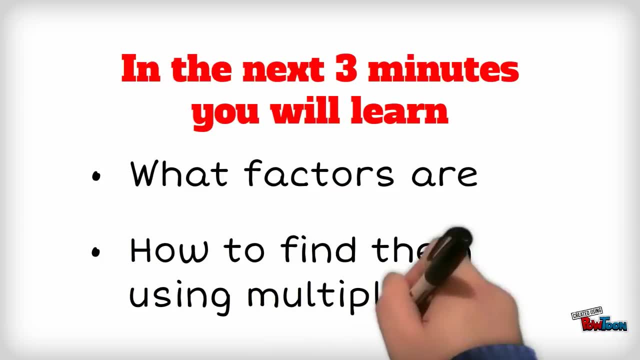 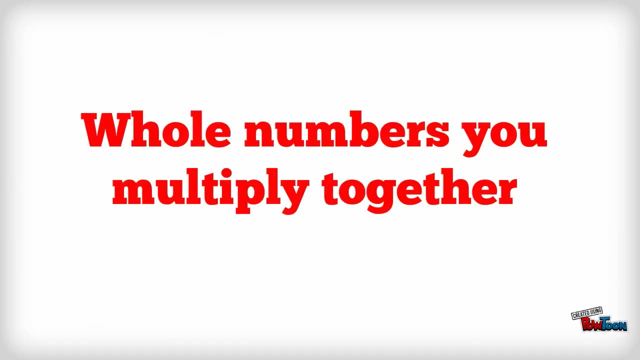 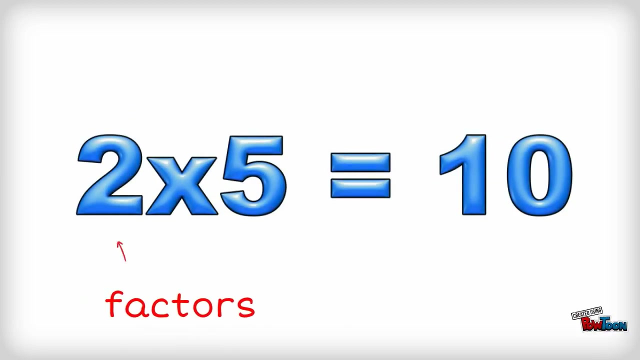 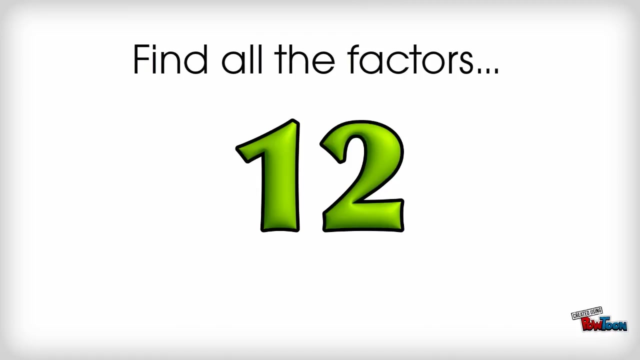 Factors for the first time, You are told to list all its factors. You could just think of any numbers that multiply together to give 12 in this example. But a better plan is to use the same simple way every time. Take a look: The first thing you do is find the simplest way of multiplying to 12. 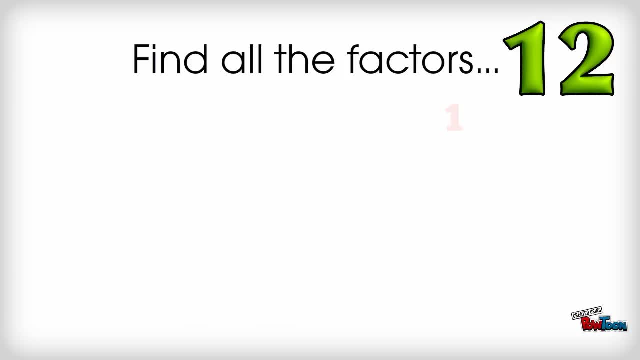 and you start with 1. So 1 and the number itself are always the first factors you list. Write the factors down in pairs 1 here and 12 over here. We will fill in the space between with other factors as we go along. For each factor pair, use an arc. 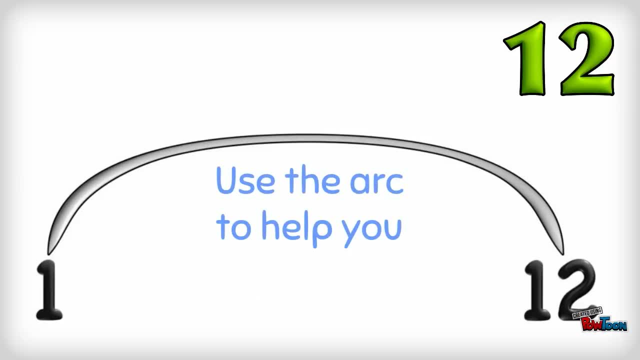 to show which factors multiply together. It helps keep your thinking clear and stops you from accidentally forgetting to write a factor down. Now you try 2 x number to make 12. Well, 2 x 6 is 12. List the 2 and the 6 and put the arc in. 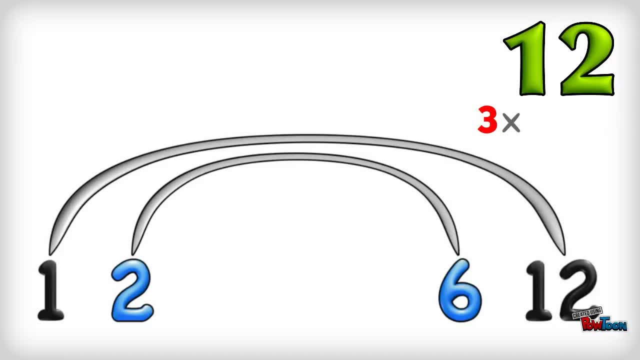 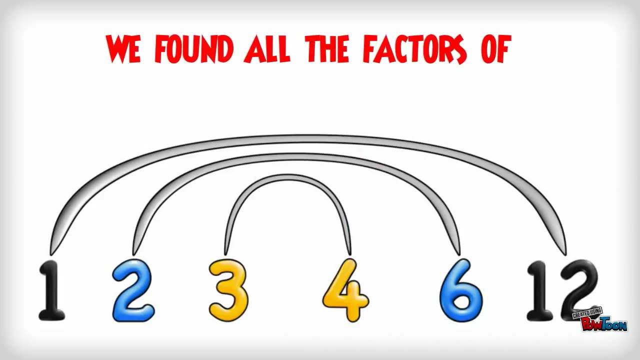 Then 3 x a number, 3 x 4 is 12. List the 3 and the 4 and put the arc in. 3 and 4 are consecutive numbers. So we know we finished, because there is no whole number between those two. We've just found all the factors of 12. 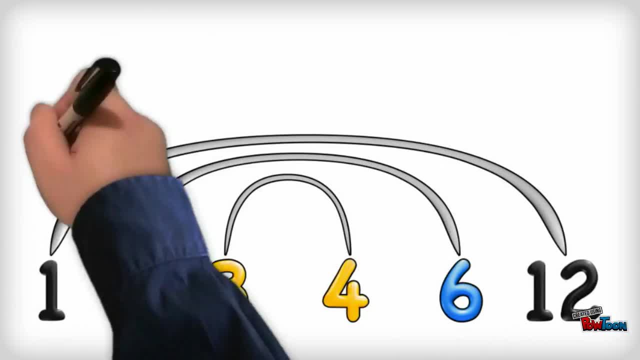 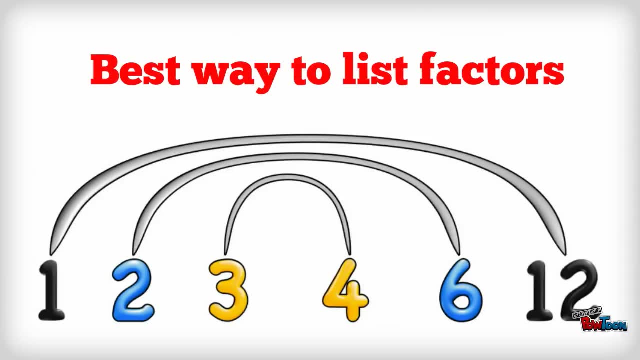 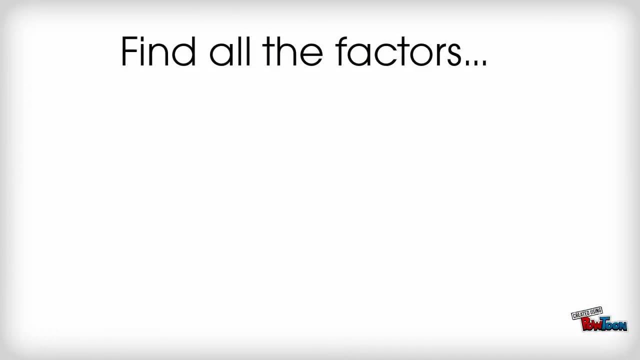 Notice that, because we worked from the outside in, the factors are in order. This is the clearest way of showing all the factors of a number and using the arc for each factor pair shows your thinking. We'll do one more example. We'll find the factors of 16. 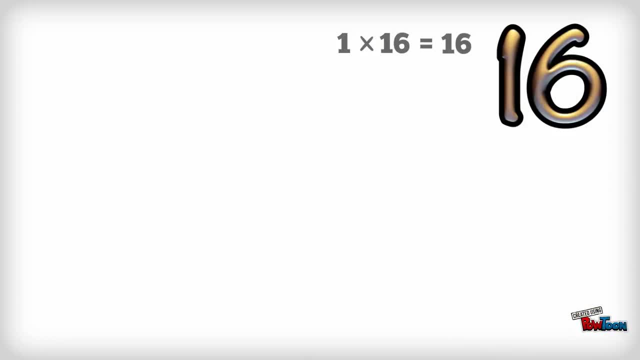 Start with 1 and the number itself, 1 and 16, use the arc. Now go to 2. 2 x a number. Well, 2 x 8 is 16. What about 3 x a number? Is 3 a factor?